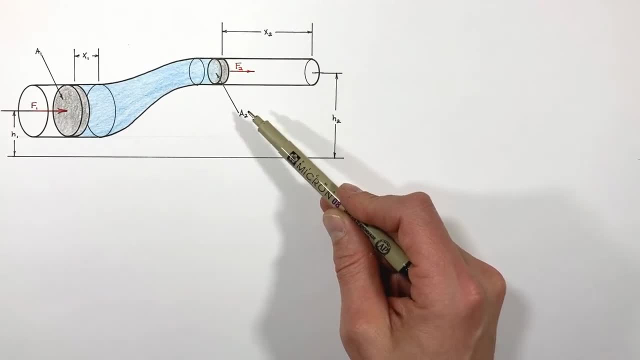 greater height and the area or cross-sectional area of that pipe is different. Now, if you look at 10 different videos on Bernoulli's Law on YouTube, you're going to find this picture- at least 9 of those 10 times. What I want to do is go through and explain this in a little bit. 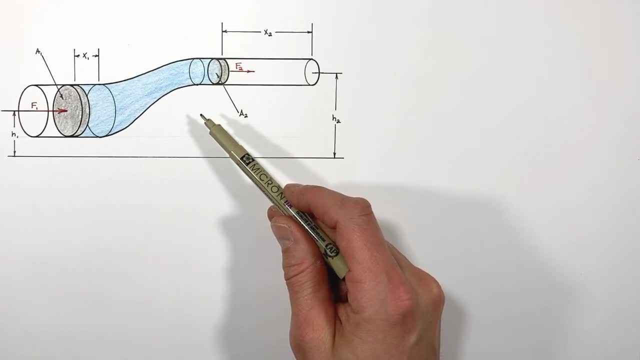 different way because, let's be honest, if those other videos worked, you wouldn't be watching this video, So let's get started. So to start our understanding of Bernoulli's Law, what I want to first look at is the work. 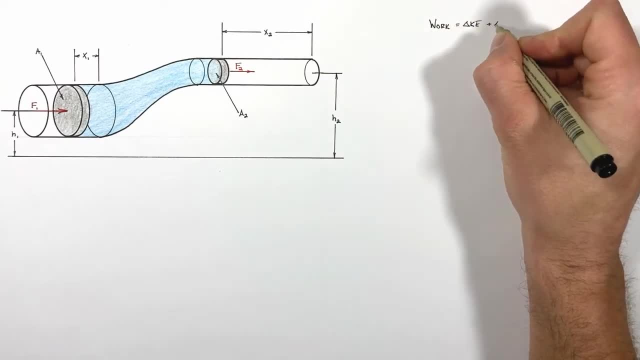 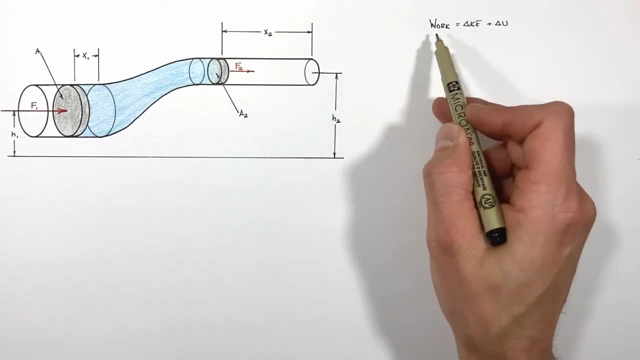 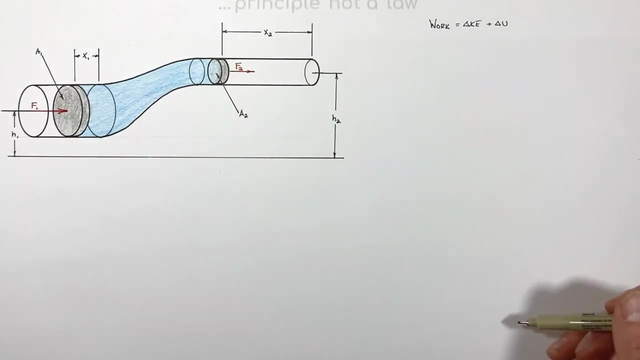 energy theorem, where work is given by the change in kinetic energy plus a change in potential energy of some particle or some mass. Now realize, all we're going to do is apply this to the situation and what will pop out down here is Bernoulli's Law. Now, if you've seen any of my 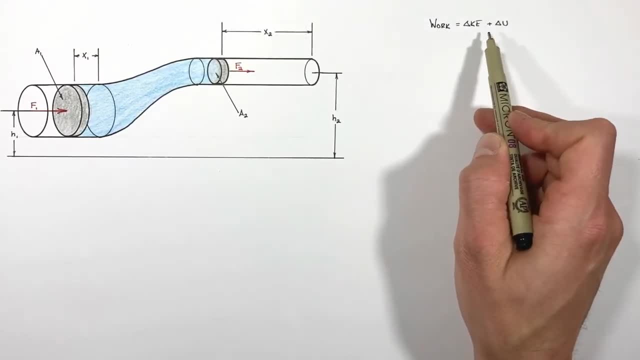 other videos in the past. I don't really like looking at the work energy theorem like this. I prefer to look at it like this, So I'm going to look at it like this. I'm going to look at it like this. I'm going to look at it as an initial and a final state within a system. 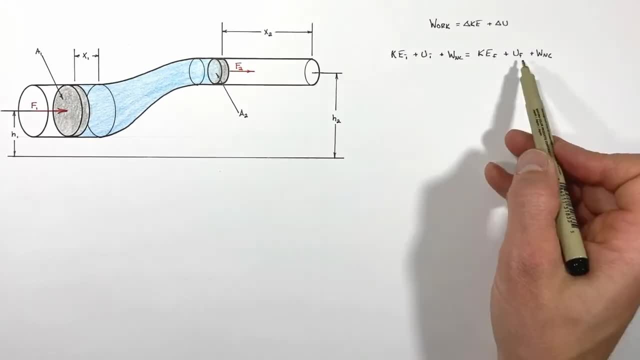 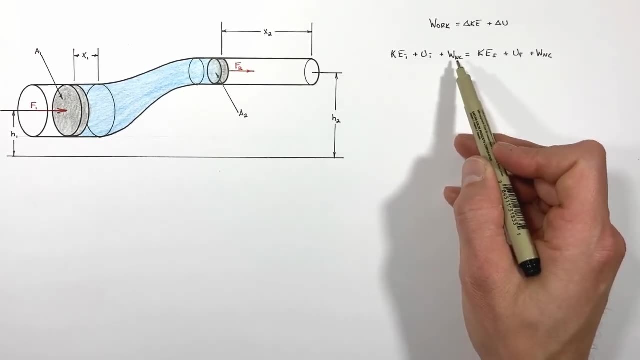 Or we have initial and final kinetic energies, initial and final potentials, and then we have these non-conservative work terms, That is, work being done on the system by any sort of outside force, In this case our force acting on this piston and our other force. 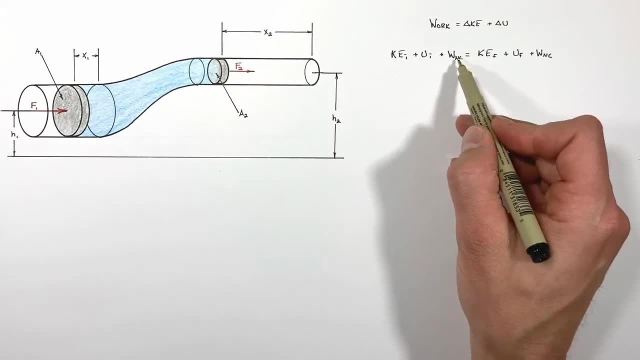 acting on or by this piston over here. So we've got work really into the system and work out of the system, And it's this idea of work that gets lost in how most people present Bernoulli's equation, And so that's what I want to go through today and really drive home is what happens with 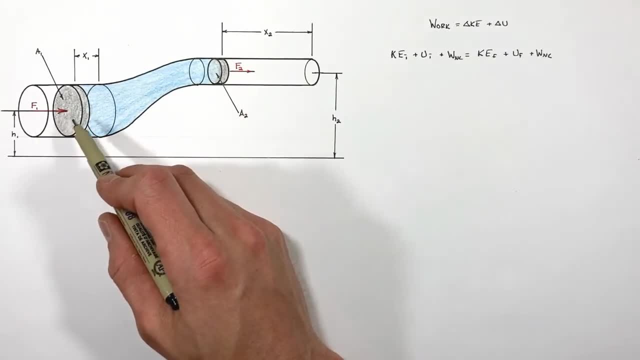 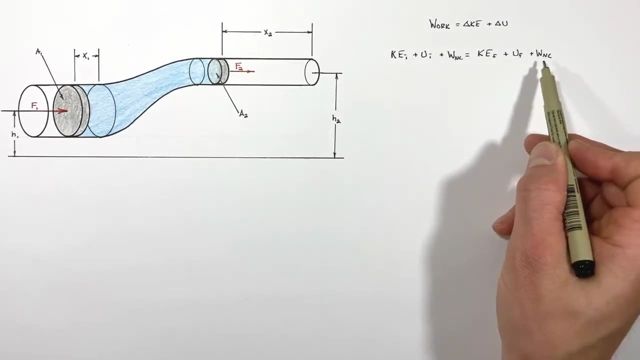 this work and how it relates to something referred to commonly as pressure energy. So to turn this into Bernoulli's law, what I want to do is look at each term individually. So let's start with the initial kinetic energy of some particle within this fluid. 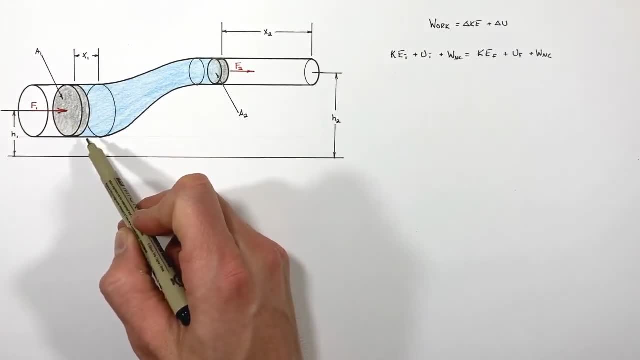 If we push on this piston and cause this piston to move forward at some velocity- we'll just call it v or v1,, v initial, whatever you want- That particle is going to be also moving forward at that same velocity, v, So that particle of mass will have some kinetic energy. We're simply going. 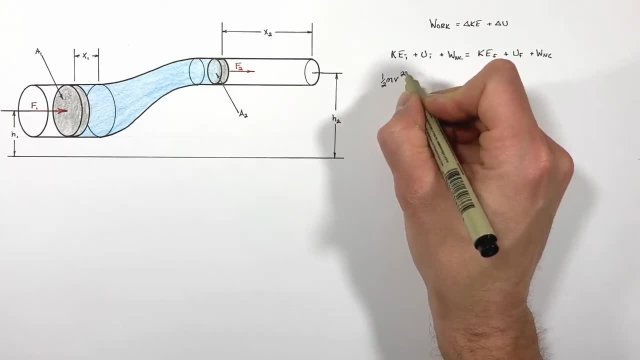 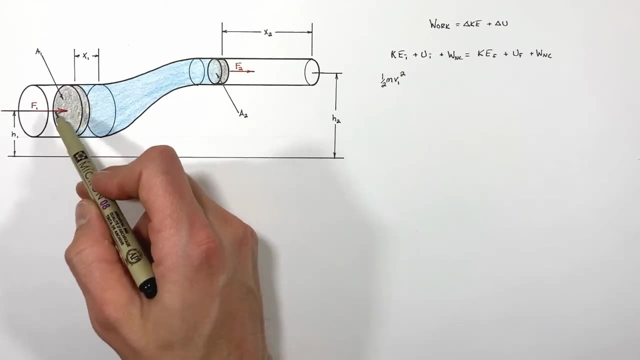 to call it one half mv squared. I'm going to call this v sub one. That is the velocity over here, at point one or on the initial side of this system that we've drawn here. Moving on to potential energy, that particle or mass of fluid has some height. We've given that. 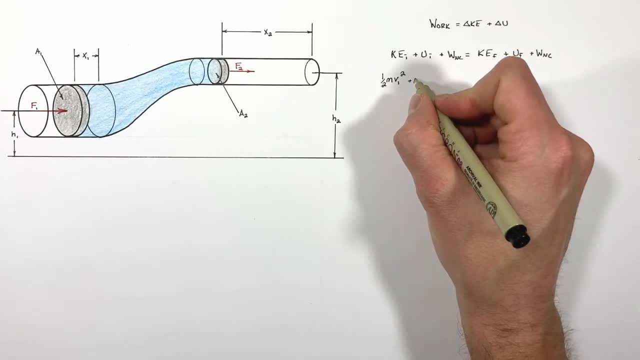 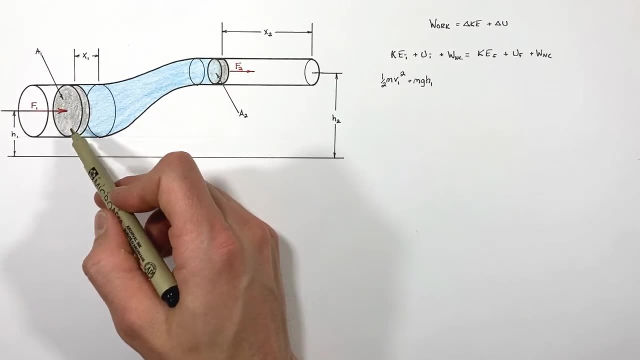 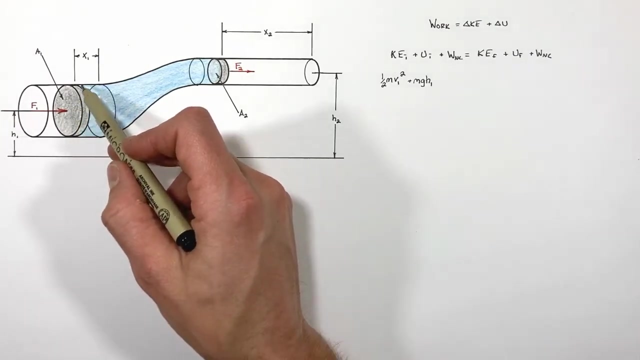 h1. And so its gravitational potential energy is simply going to be m times g h1.. Now, as the particle is pushed forward by this piston, which has some force on it, we're going to do some work on that particle or on that fluid in front of the piston. So if we look at all the fluid in front of 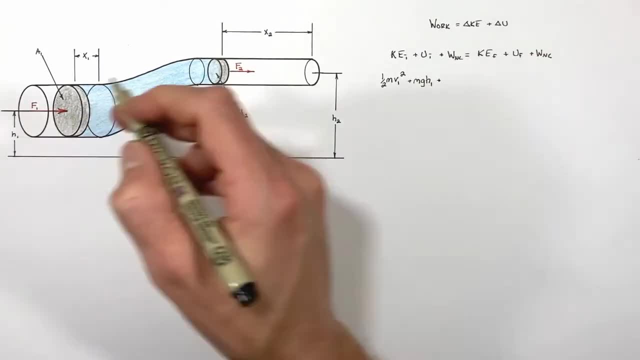 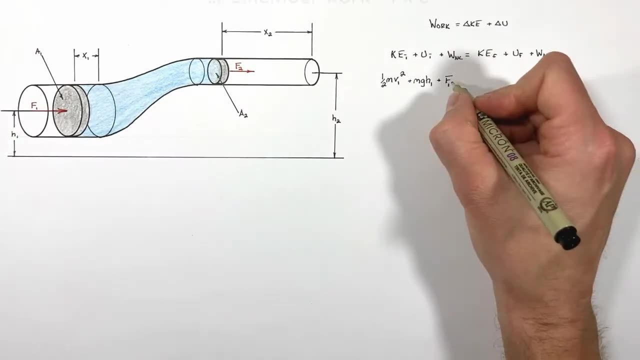 the piston. ultimately, what's happening is there's some force on it And so we're going to do some work, And if we look at this только in liquid, we can see that there's this total force, F- or really F- at position one which is going to act over some distance. I'm going to call this x one. 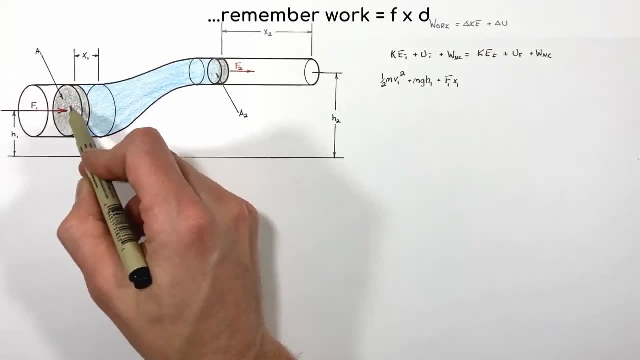 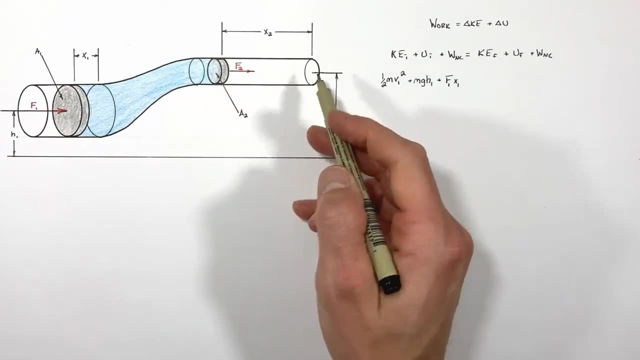 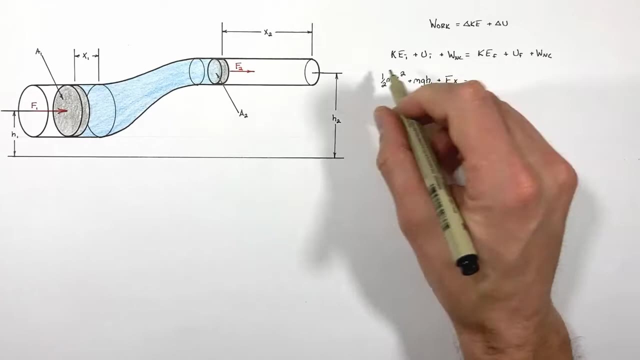 Really, this is work done on this piston or on the fluid immediately in front of the piston. Moving to the output side of this system, we have almost the same exact thing We're going to have. this piston gets pushed forward by this fluid and therefore it moves, So it has some kinetic energy. 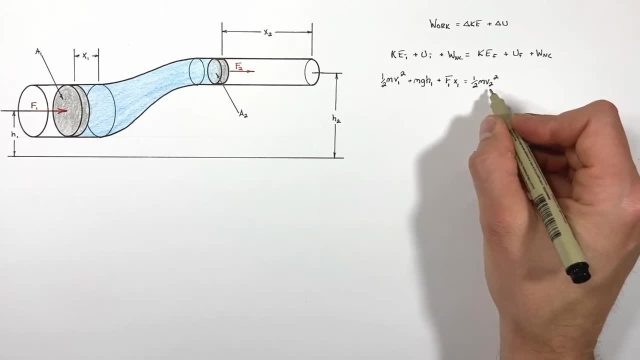 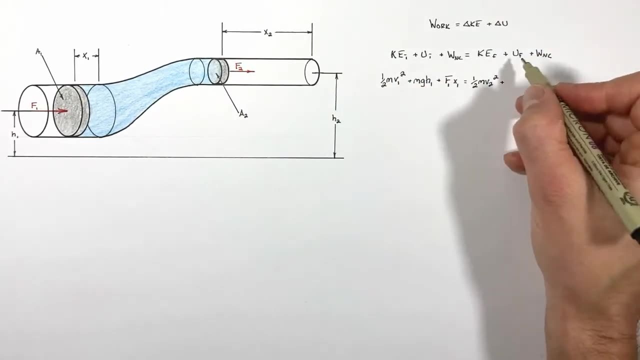 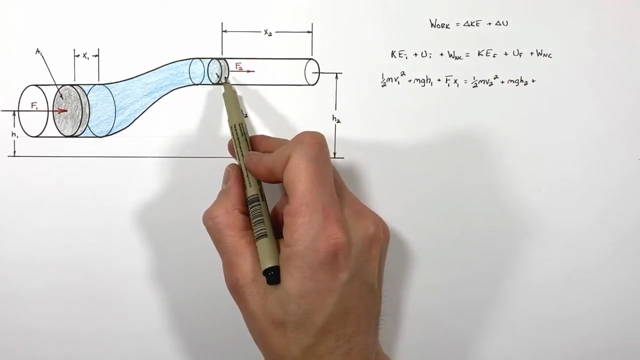 I'm going to call that 1 half mv squared with v sub 2, because that's the velocity up here at point 2 or on the outlet side of this system, plus our final or outlet side potential. that's going to be mgh plus the non-conservative work done at this piston. so that is going. 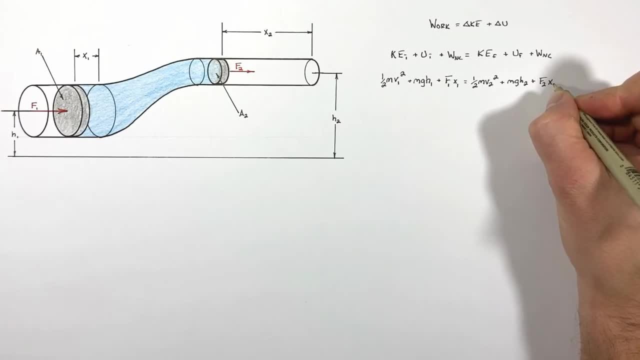 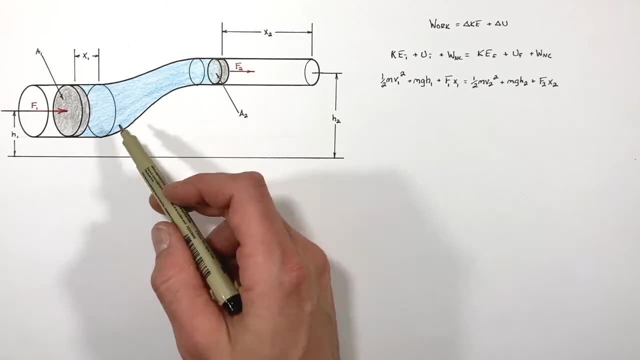 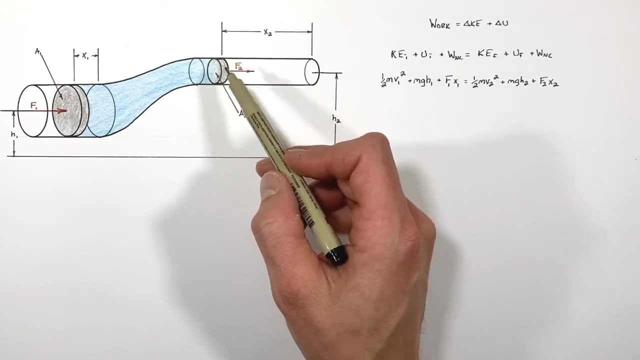 to be f2, x2.. Now, one thing that is tempting in this problem is to go through and say that we're going to apply Pascal's law, and that is to say we're going to treat this like a hydraulic system where we have an input and an output cylinder, and we can't do that in this problem, I know. 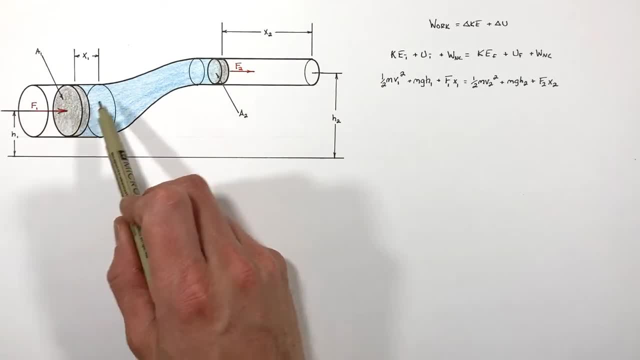 I've drawn pistons here, but ultimately what happens is, once we start moving these pistons fast enough, there are shifts in pressure in this fluid as these pistons move. so we cannot apply Pascal's law and treat this like a set of hydraulic cylinders. Okay, 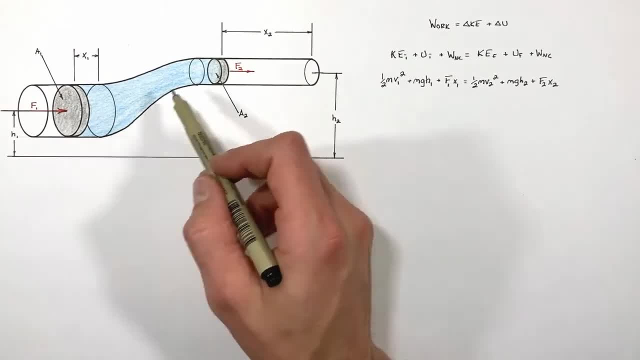 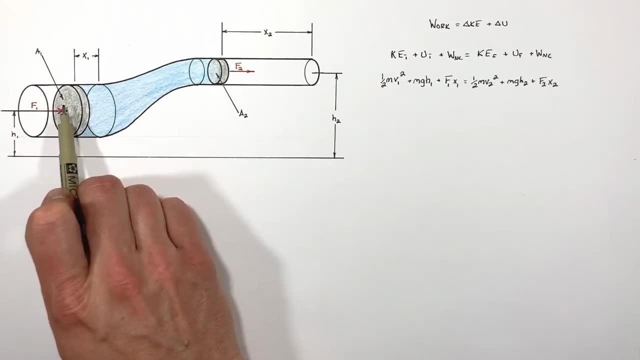 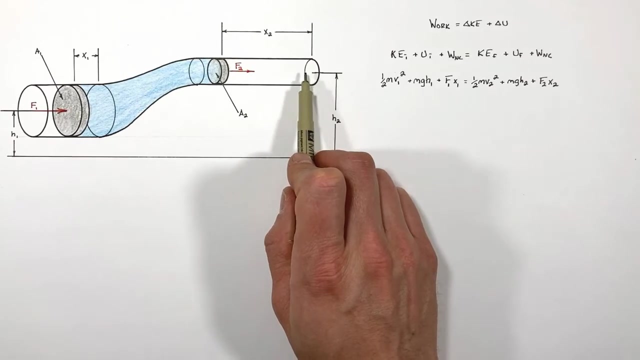 But what I do want to apply in this problem is simply the continuity equation, and that is to say that if a certain volume of fluid or mass of fluid is pushed forward by this piston here, that same mass or volume of fluid is going to be pushed forward up here. 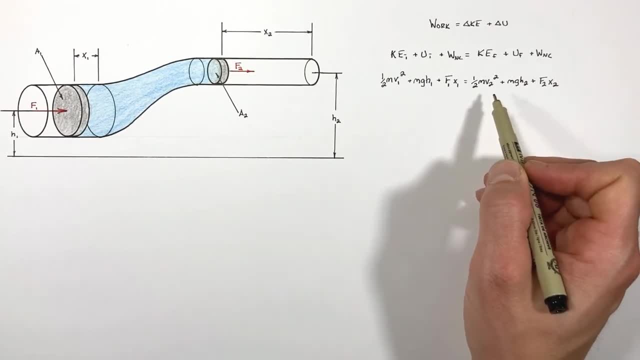 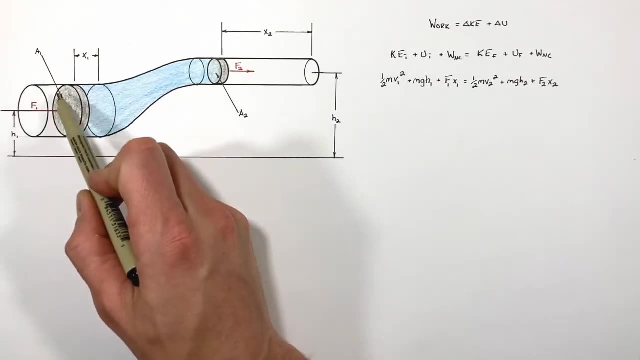 Now to take this equation, which is largely just based in general physics, and to start to apply it to fluids and Bernoulli's equation. what I want to do is take this basic idea of a force Which is acting over an area of a piston and convert that into pressure. 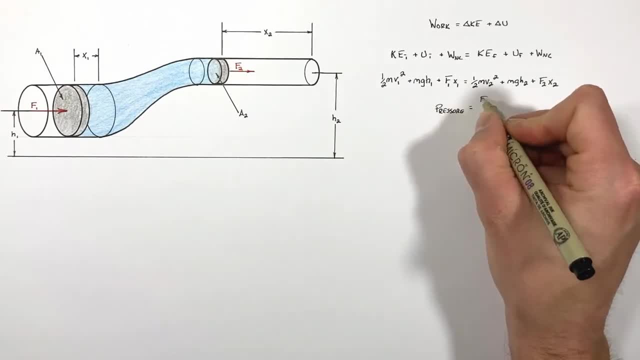 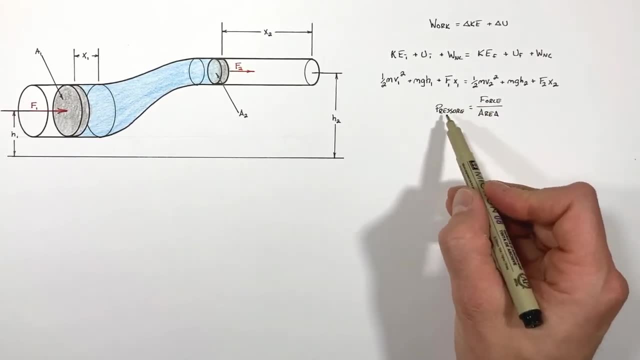 Now, you'll remember, pressure is given by force over area, And so what we can do is we can take this pressure term and substitute it in here and here where we have force or work being done on the fluids. Now, you'll notice, If I was to stop right here, what I've done is I've divided this term by a one, and that's. 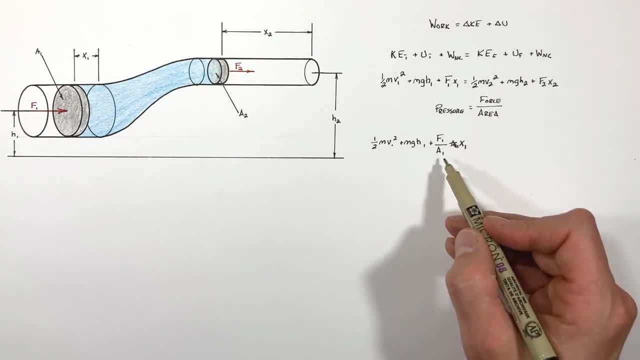 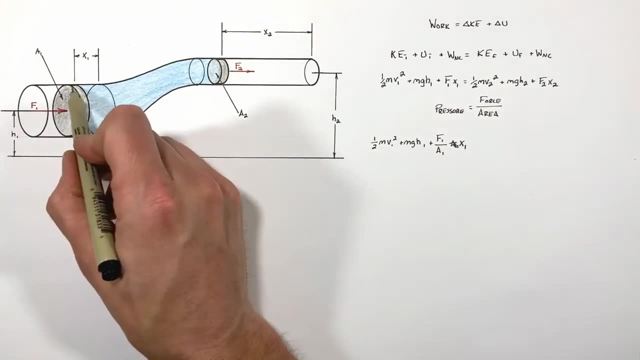 not okay. We can't do that, just interjecting or deciding to divide one term by area. that that's illegal math. So what I'm going to do is I'm going to take this, this x one, this distance which we're going to allow this piston to move forward, and we are going to multiply it by one. 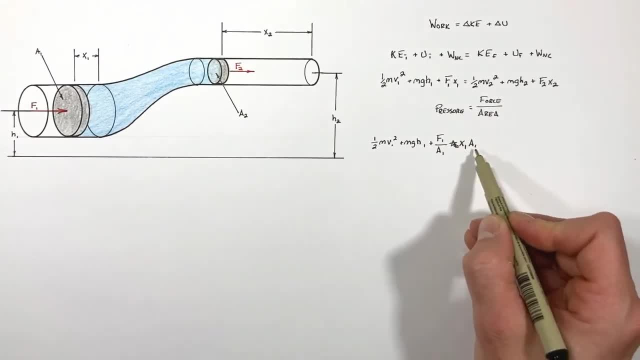 So, ultimately, you'll see, I've divided this term by a one and multiplied this term by a one or area, and so I haven't committed any sort of illegal math here, But we're going to be able to rewrite this in a very useful way in just a second. 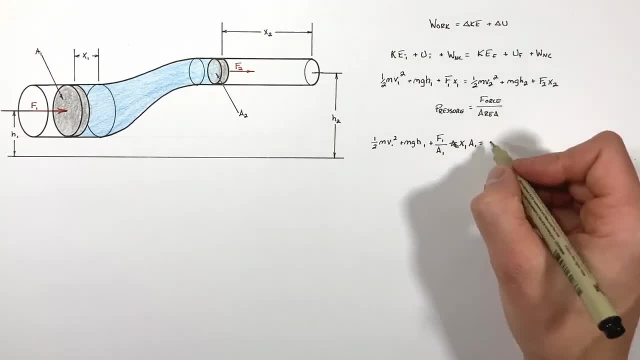 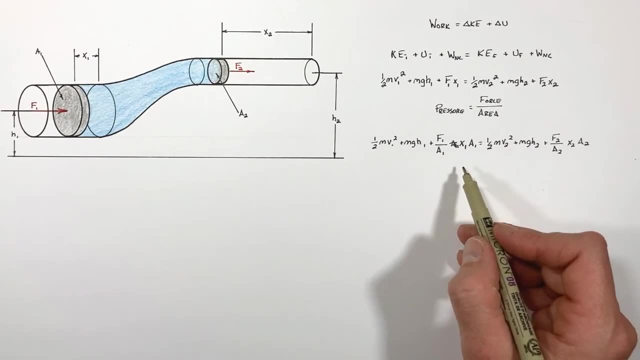 So writing out the right half of this equation, doing a similar sort of substitution. Now, the way this sits, you could actually look at this as Bernoulli's equation, but it's a little bit useless this way. So what I want to do is look at this term- f over a- as pressure. 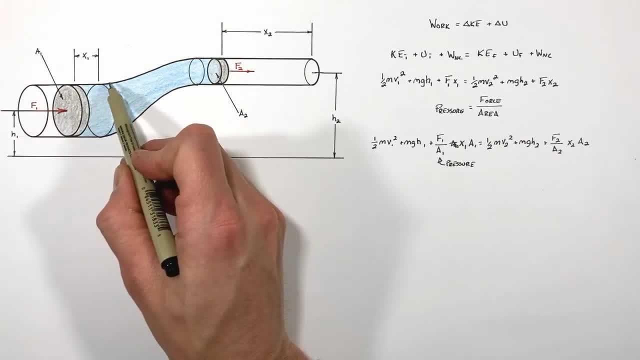 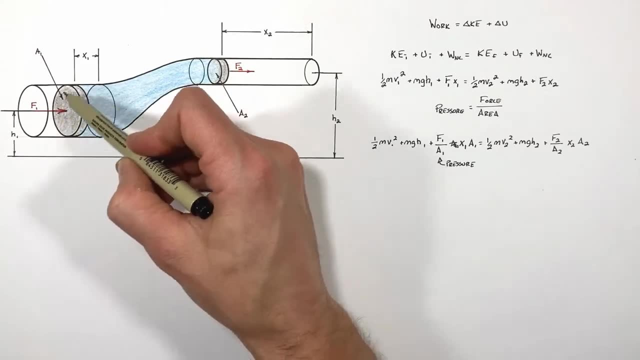 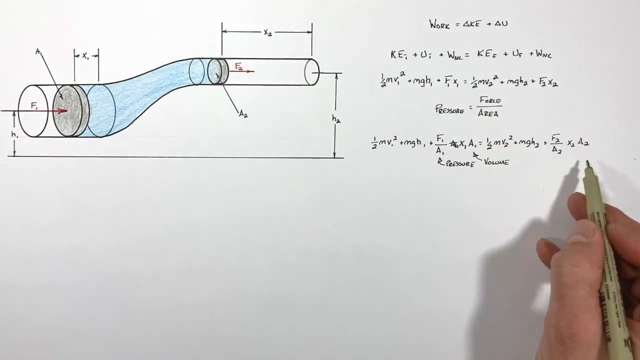 I also want to point out that this position or this length- Which this is Right- The piston is going to move through the cylinder or two, multiplied by the area or cross sectional area of this piston, is a volume, And when we rewrite this equation, we get: 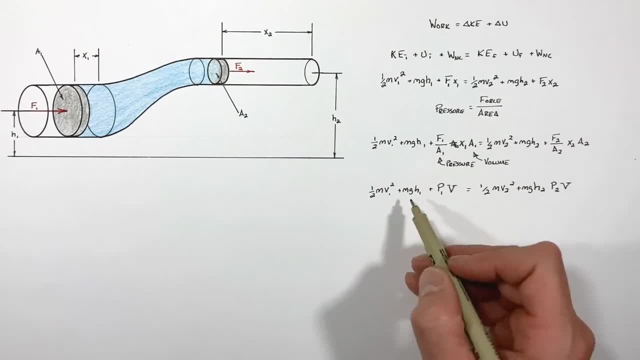 Now the first thing I want to point out with this is we've got to be really careful, especially if you're sitting there taking notes on this stuff, writing it down. Be really careful about the difference between v for velocity. I'm showing that as a small v. 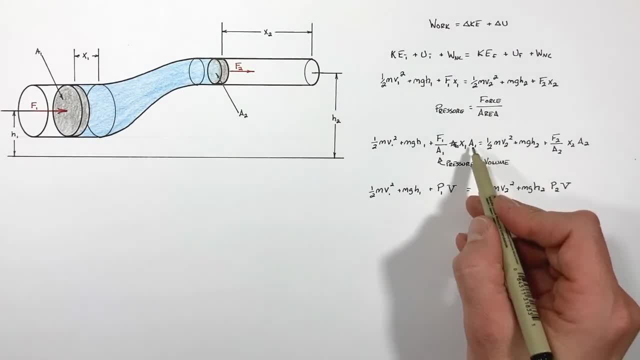 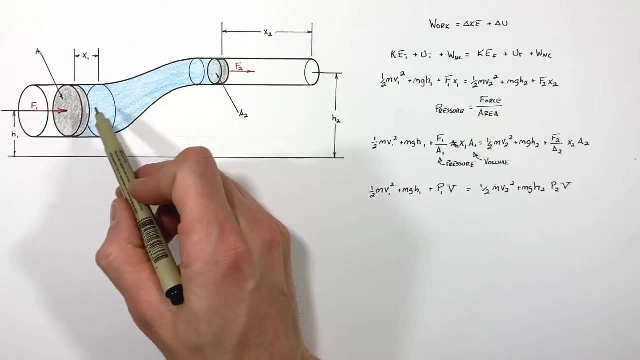 Versus capital, V for volume, like we came up with here. Now, going back to some assumptions and constraints that I talked about earlier, we said we couldn't apply Pascal's law, that is to say, the pressure in the fluid down here is going to be different. 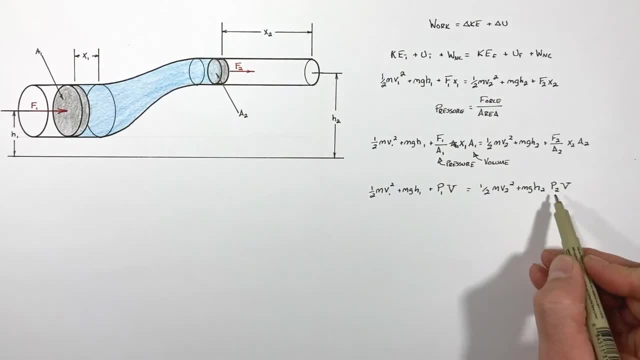 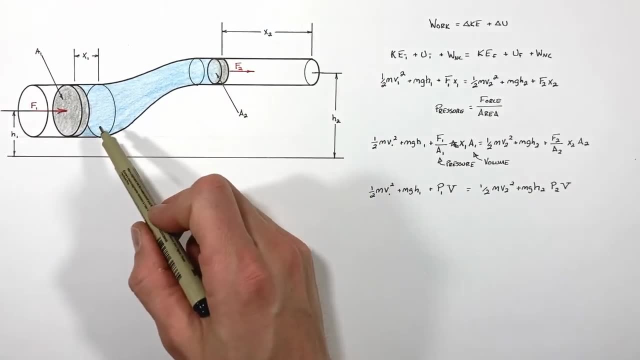 than the pressure in the fluid up here. So I have a pressure here which is different from the pressure here. you can see p one and p two, indicating the pressure is different at the two points. However, we are applying continuity to this problem, That is to say, 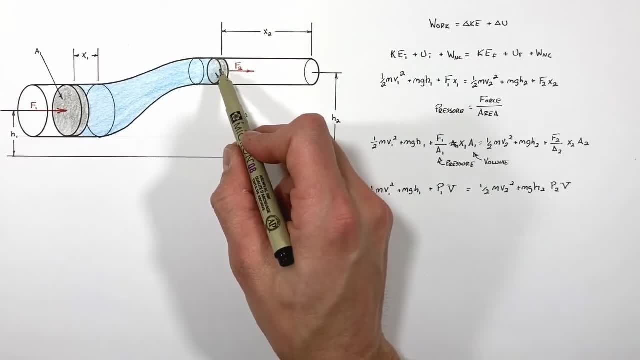 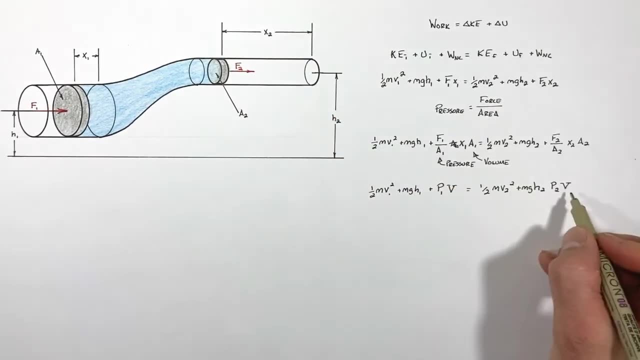 That is to say, the volume of fluid pushed by this piston is equal to the volume of fluid accepted or that is going to push this fluid and piston forward. So our volume isn't v sub one and v sub two, it's just v the volume that is pushed by the system. 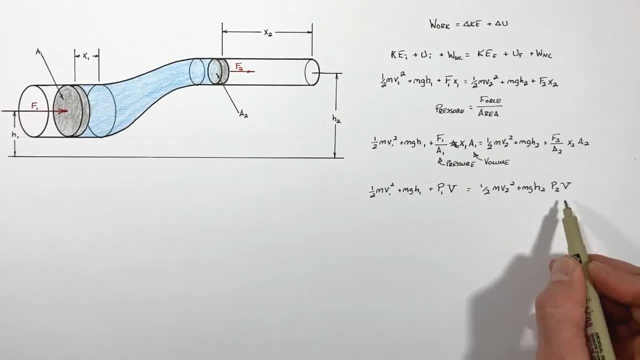 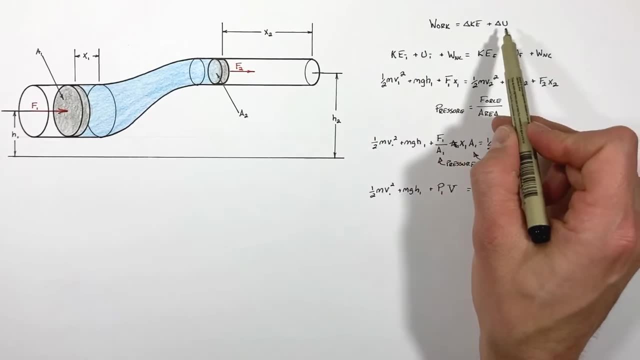 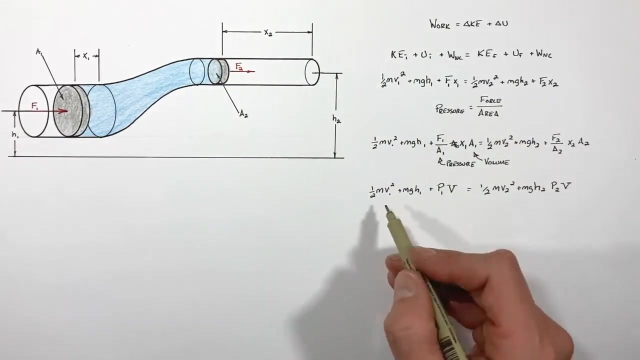 Now this is the point where I want to stop and talk about what's going on here and get at some misconceptions that occur when talking about Bernoulli's equation. Really, all we've done is we've taken the work- energy theorem, The conservation of energy- and then applied some pressure to this and made it somewhat situational. 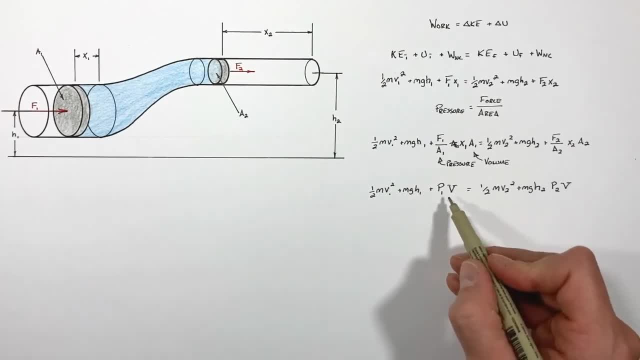 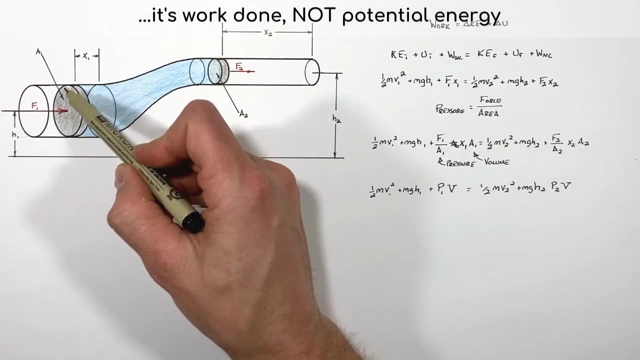 We've still got kinetic energy, gravitational potential, and then there's this term and people try to call this pressure energy, and while it is in fact referred to as pressure energy, I want you to realize this is really the work done. These pistons make the system look as though this. this system starts here and ends there. 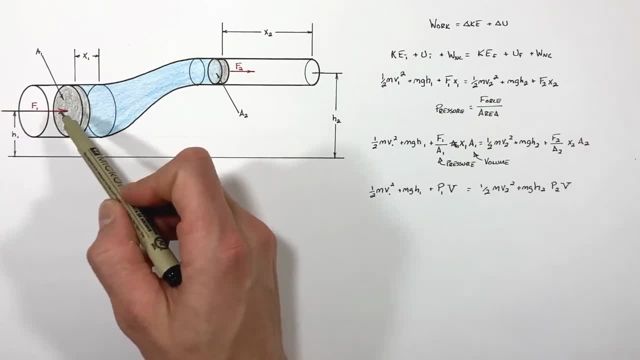 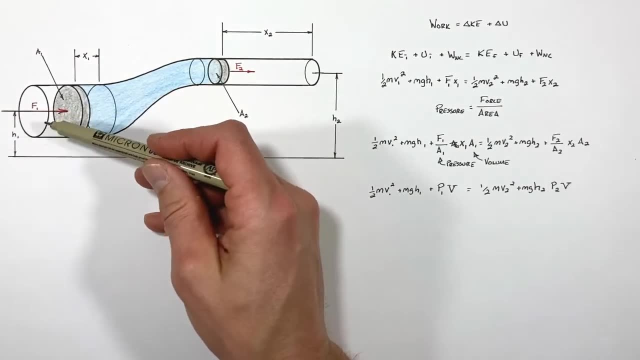 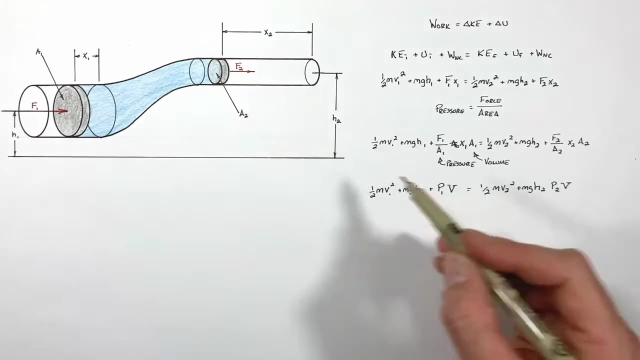 But I want you to realize there's. there's some input Force here. there's energy coming in from the outside world. now, even if we remove this piston and we have fluid move on to the left here forever. at some point something has to be doing this work on this fluid and transferring pressure into the system. 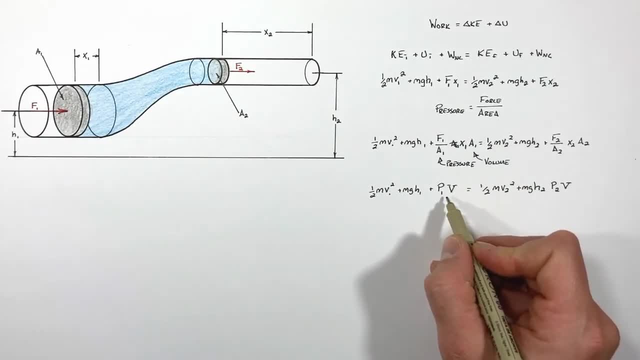 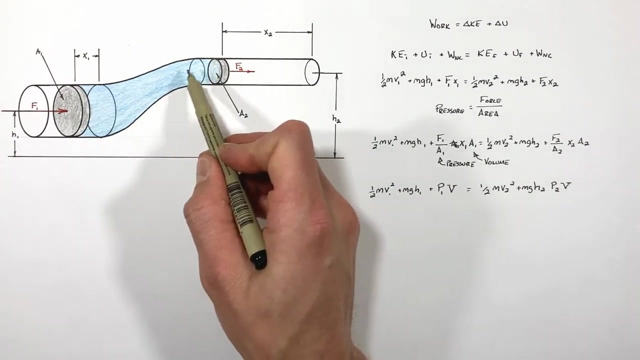 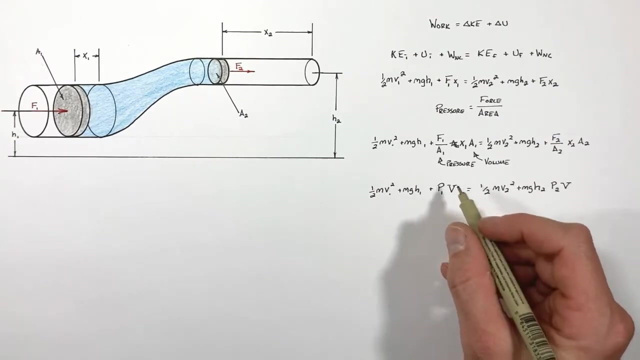 And so, ultimately, what this term is, you can think of as work done on the system or input work, and over here we have what is ultimately output work. There's work in and work out. It all just boils back to the work Energy theorem and the conservation of energy, and that gets lost when people refer to this as pressure energy, and seeing people go so far as to say that the units of this are Jules- which they are, mind you- and try to reference the ideal gas law. but if we're talking about an incompressible fluid here, trying to talk about the ideal gas law with this is a little bit strange, because think about it. 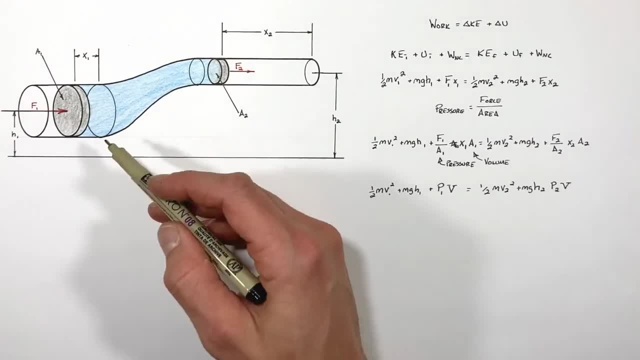 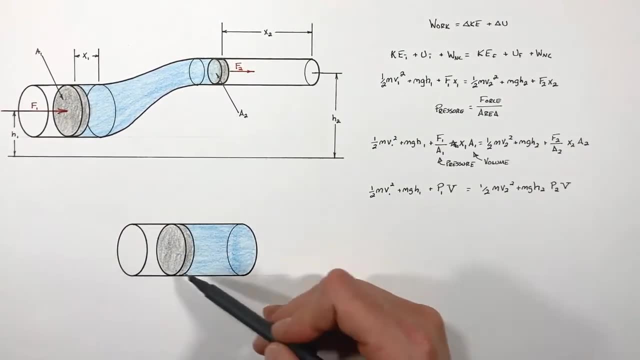 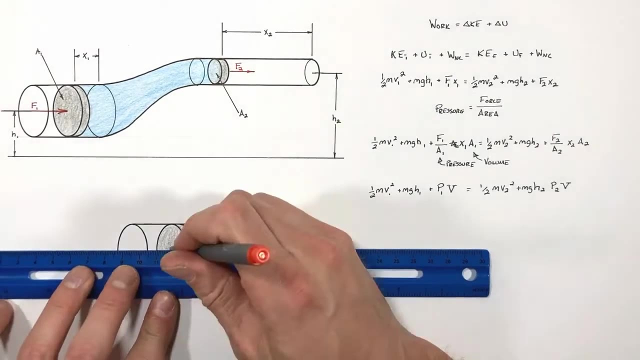 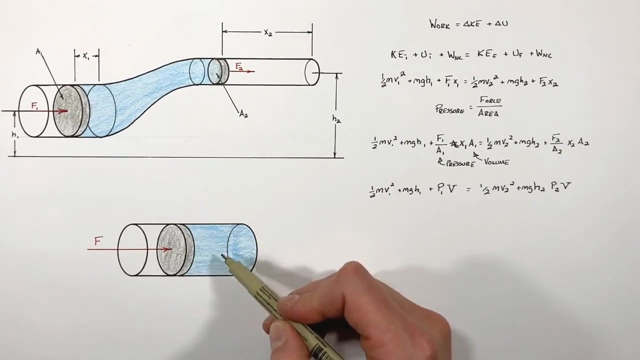 Imagine we took a confined, incompressible fluid Like, say, water inside a cylinder. if we were to take a piston into, push on that water with some force against this piston, I don't care how hard you push against this piston, if this is an incompressible fluid you're going to do no work. as you push against this piston, you can make as much pressure in this fluid as you want, with as much volume in this fluid as possible, but it is not an 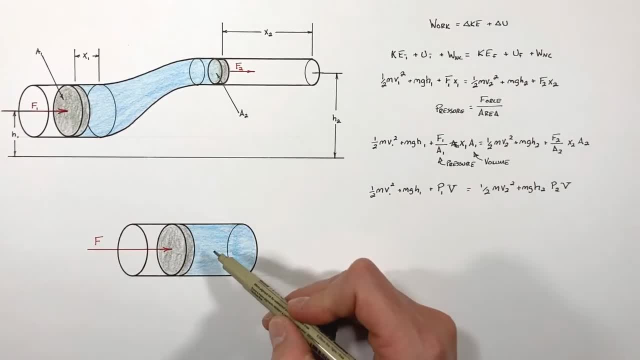 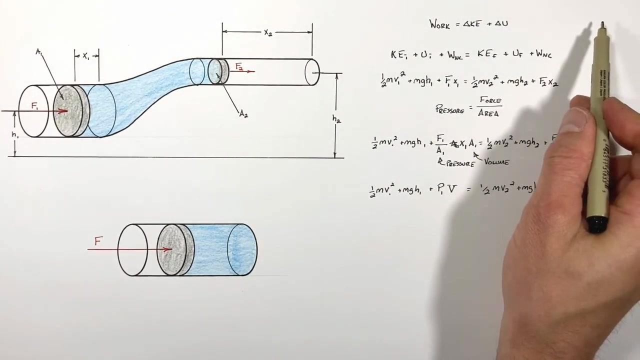 A Negotiable, you will do absolutely no work on this fluid, And so it's this idea of pressure times, volume is energy that can be a bit misleading. Now, yes, if this was filled with something like, say, air, and we were to push against this piston, really, all we've done is we've created an air spring that air would compress and it would store energy, and I've got a video explaining the math behind all of that exactly right here. 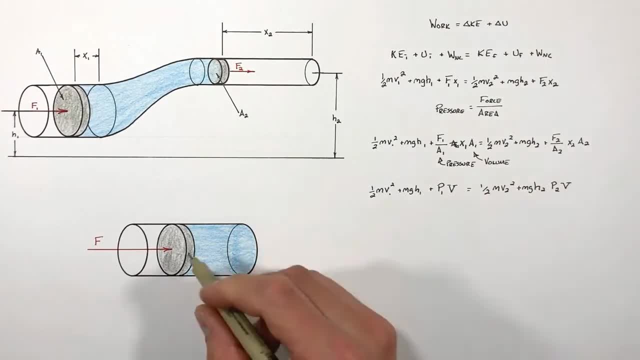 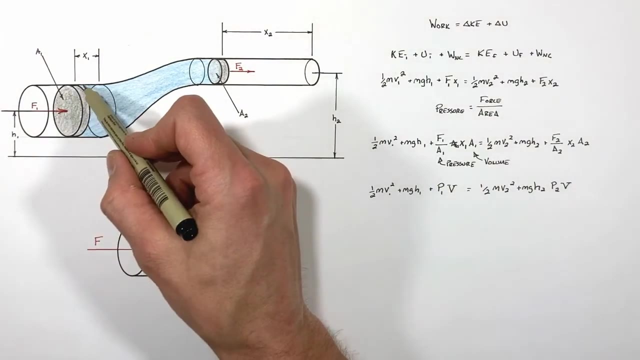 But the point is, I don't want you to think that this pressure Times volume is some sort of form of energy which exists within the fluid. it is work done on the inlet and worked on on the outlet side of this fluid, or really the work done prior to some point we're looking at and after some point we're choosing to look at. 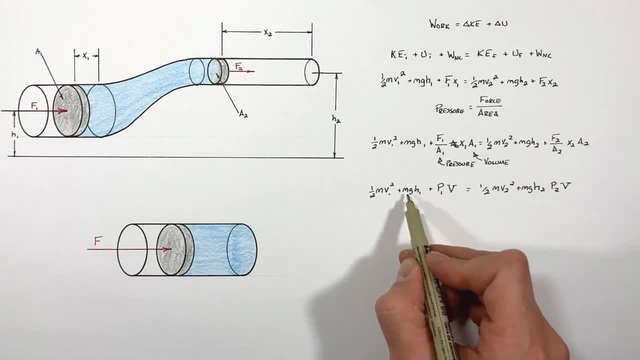 Now getting back to deriving Bernoulli's equation, you'll almost never see Bernoulli's equation represented with masses in them. What we'll more often do is what is ultimately a clever use case, And that is to talk about not the mass of a fluid, but the density of a fluid, and you'll remember, density is given by 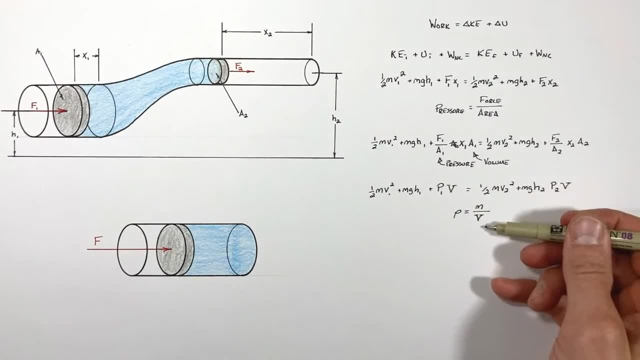 The Greek letter row, density is equal to mass over volume. So if we were to rearrange this for mass, We can substitute this term in anywhere we see mass within this equation. here And now, what we have is what seems like an impossibly long expression, but you'll notice the volume of fluid which we allow to flow through this system. now 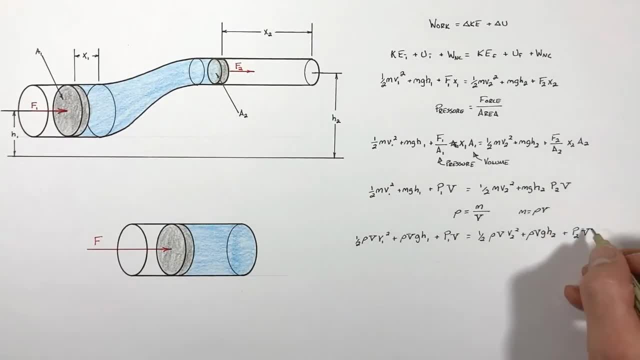 Is in every single term, and that is to say, it's going to cancel out, Which leaves us with This equation, which is often referred to as the energy form of Bernoulli's equation. What I want you to realize is the left half of this equation. 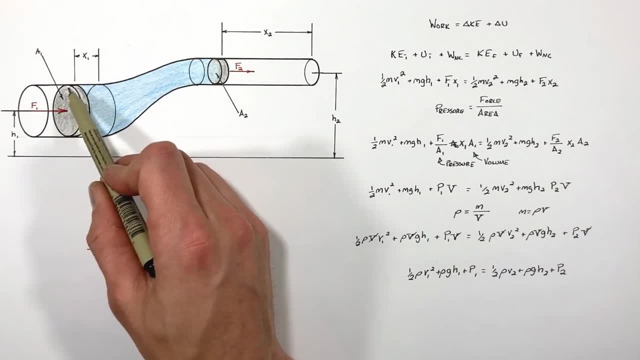 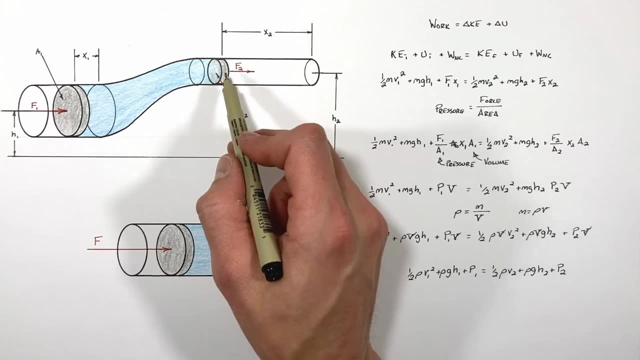 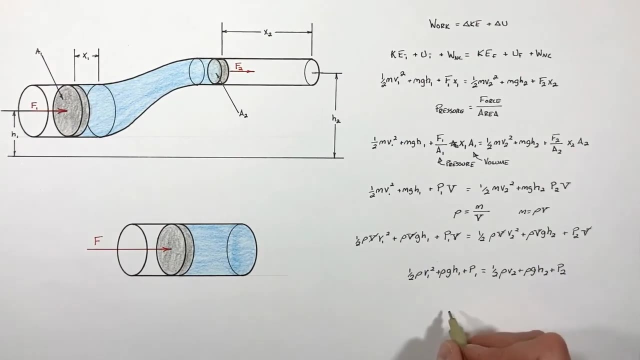 Describes the total energy content and work done on the fluid on the inlet side. here And over here we have the total energy content and work done on the outlet side. So the way we'll often represent Bernoulli's equation is not as an equality of before and after. the way you'll see it typically is given by: 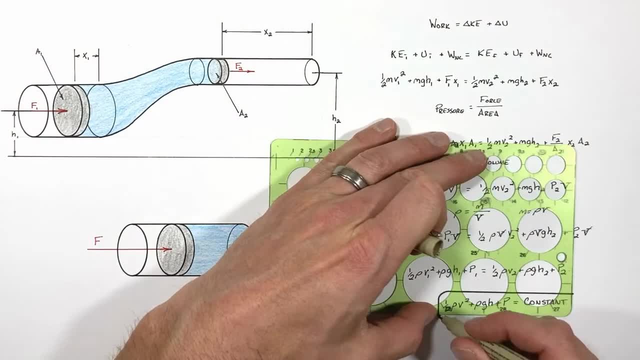 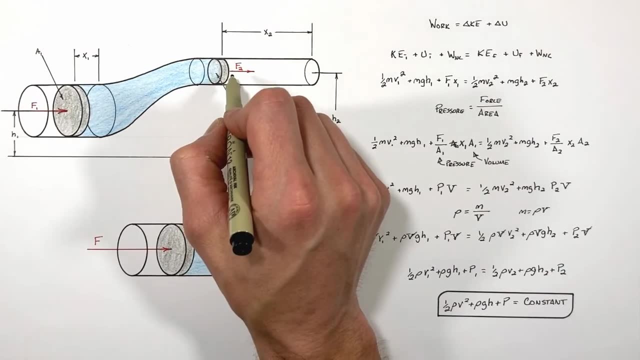 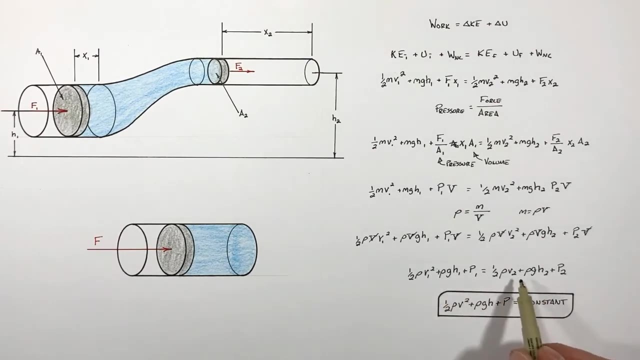 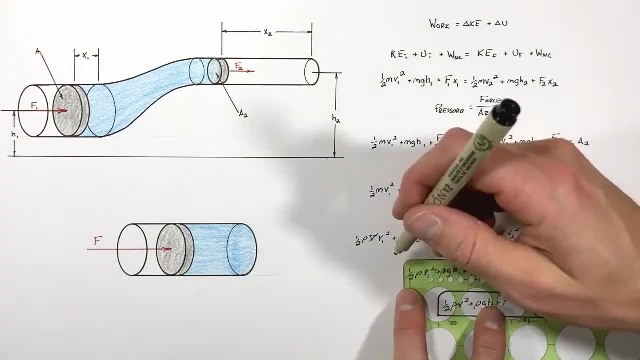 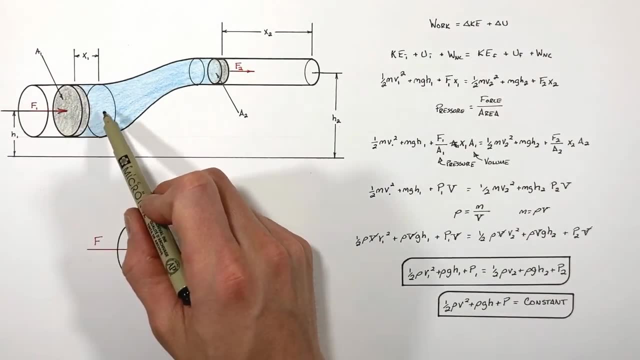 This. this is really how we're actually going to functionally use Bernoulli's equation, so I'm going to give it a box too. So this is Bernoulli's equation. What I want you to realize is it doesn't just apply to incompressible flow in necking pipes here. 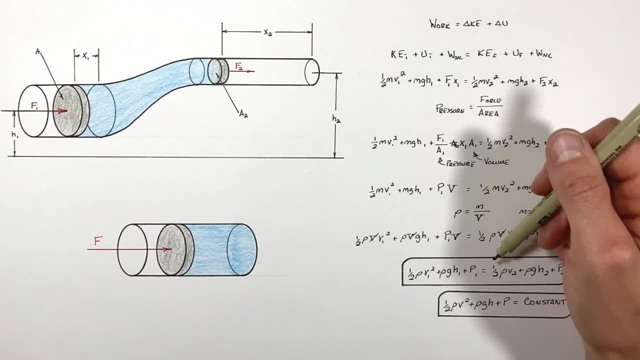 We can apply this equation, apply this equation to, say, air moving over an airplane wing. we can apply this to something like air traveling through, say, a carburetor or- yes, of course you know- water moving through a hose, something like that. there's lots and lots of places to apply this. I'm gonna get into some examples in future videos. 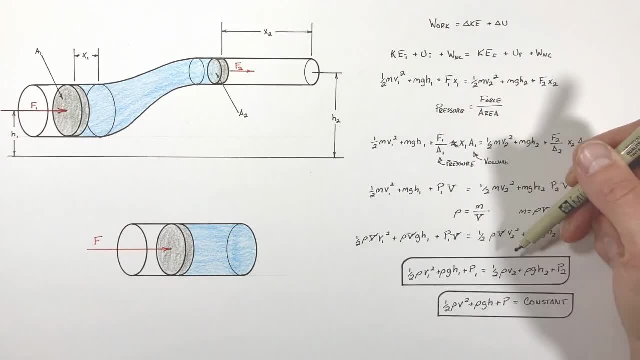 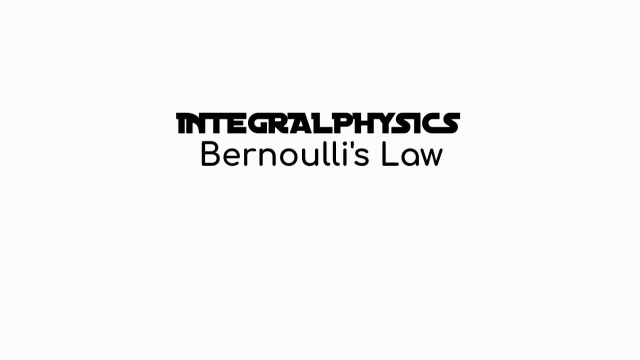 here, but this is the Bernoulli's equation and, on that note, that's all for now.